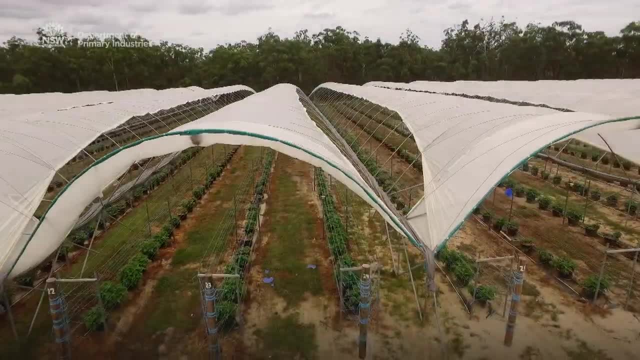 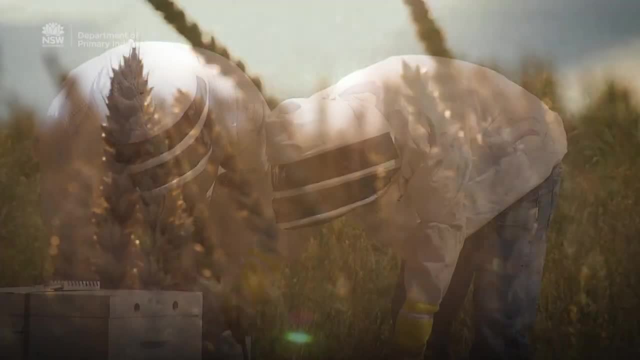 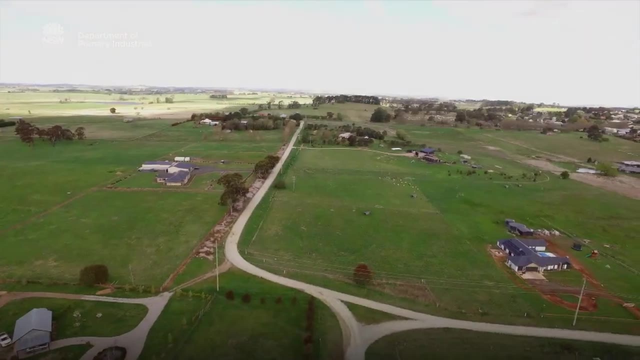 used for agriculture. These are also adapting and transitioning to the impacts of climate change. Appropriate consideration of agriculture within the planning framework is necessary to ensure a diversity of foods, short supply chains and a healthy agricultural economy. Changing community needs and aspirations can be reflected in the use of agricultural land. 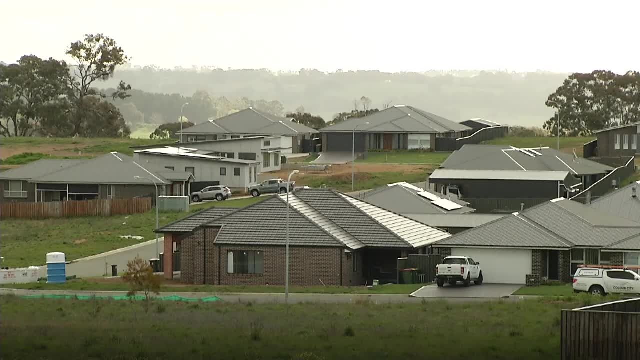 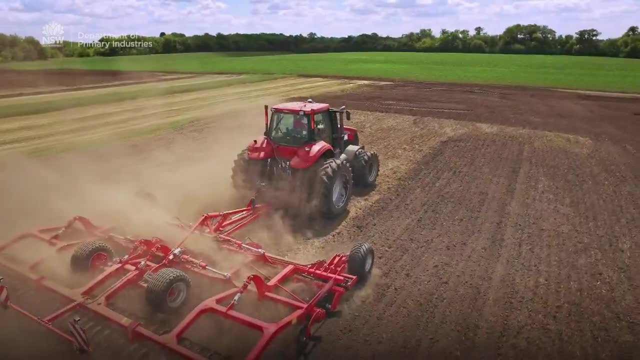 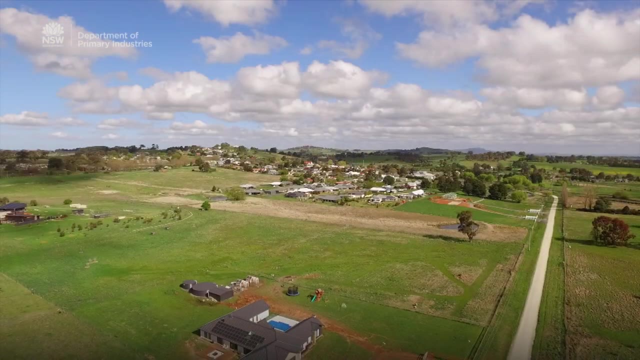 When agricultural land is converted to non-agricultural uses, such as residential or industrial uses, it pushes agricultural production further away from markets. Innovative soil and climate combinations are the key pieces of infrastructure and can fragment the rural landscape. This reduces the productive capacity of the land and makes 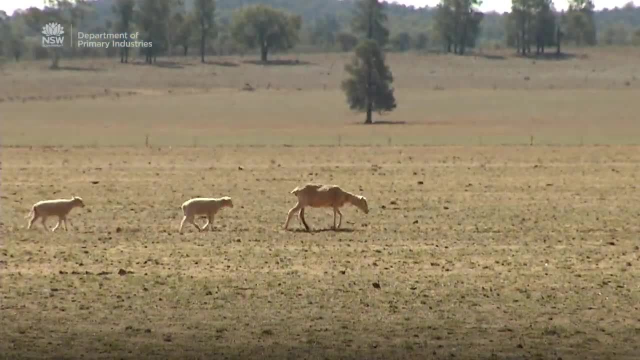 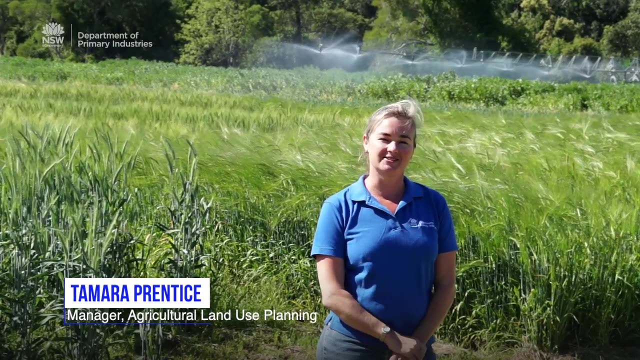 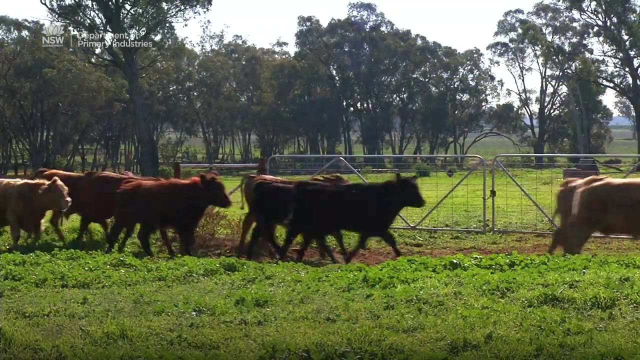 our food chains more vulnerable to shock such as natural disasters or the COVID-19 pandemic. Hi, I'm Tamara Prentice. I'm the manager of the agricultural land use planning team within the Department of Primary Industries. Our role is to ensure that agricultural industries and the land and the resources upon which these 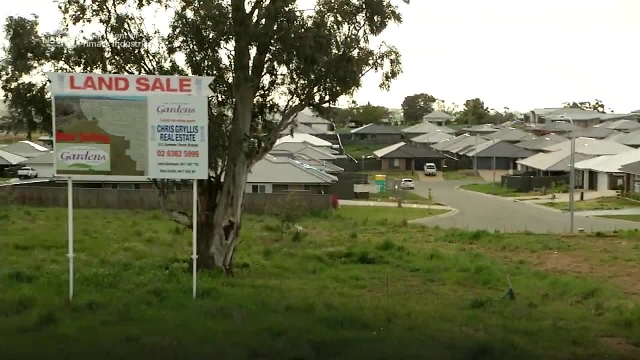 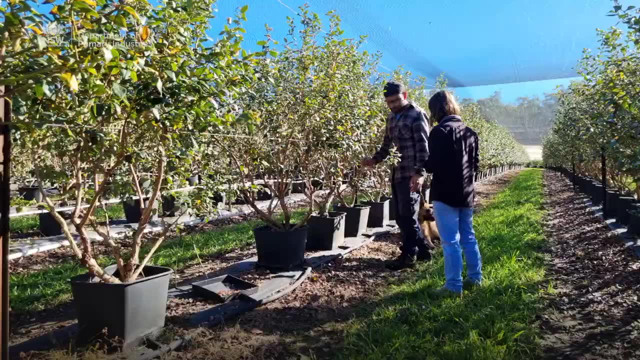 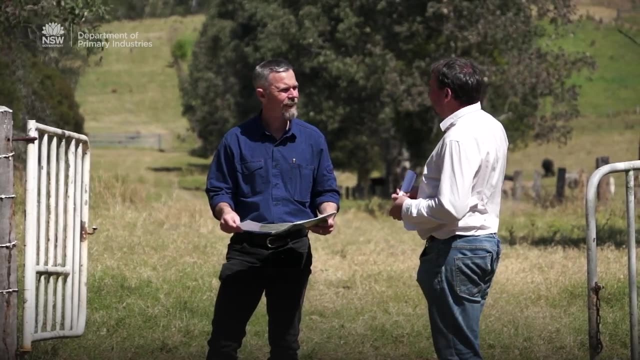 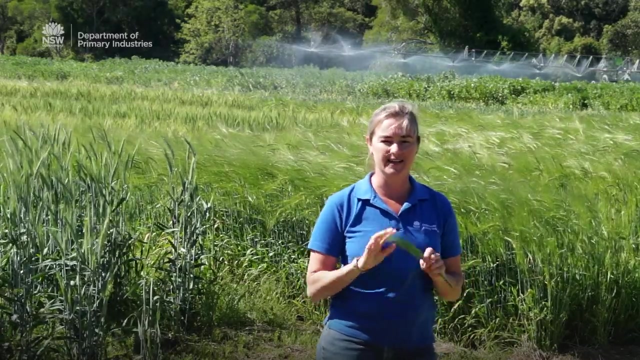 depend are protected. I have agricultural land use planning officers covering all of the planning regions across the state. Our officers have knowledge of the agricultural industry and the issues unique to their regions. They have strong contacts with council planning staff and agricultural industry stakeholders. Collectively, our team has extensive knowledge and skills in planning soils, water and environmental. 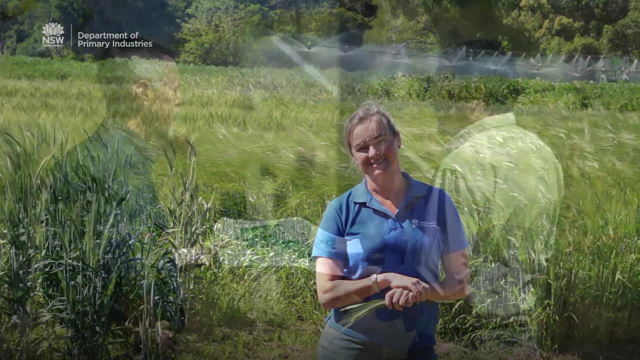 science that can be applied to agricultural land use planning matters. I'm Tamara Prentice. I'm the manager of the agricultural land use planning team within the Department of Primary Industries. The agricultural land use planning team provides expert agricultural planning advice to state. 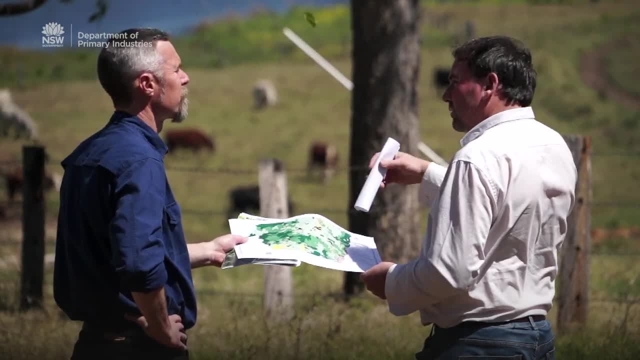 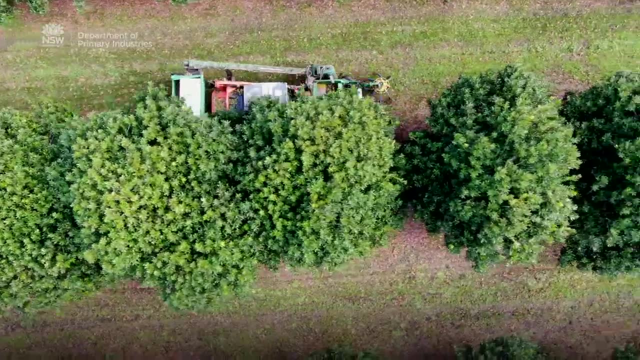 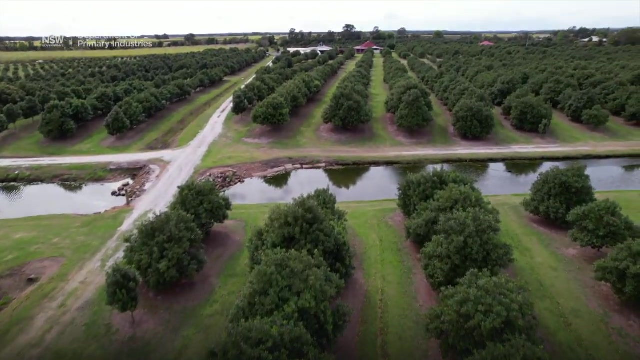 agencies, local councils and agricultural stakeholders to achieve positive outcomes for agriculture. The team supports the development and review of regional plans, local strategic planning statements and local land use strategies to ensure that agriculture is appropriately considered at the strategic planning stage and that resources important to agriculture are safeguarded. 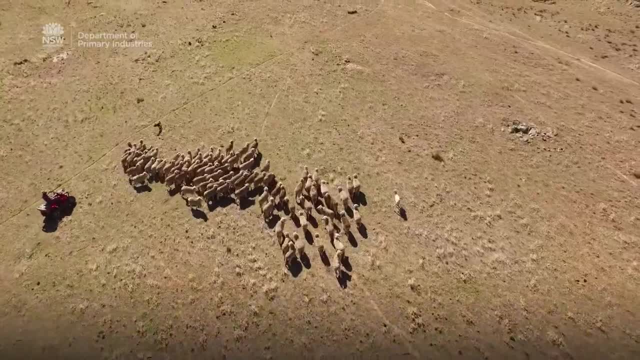 The team have built strong relationships with other jurisdictions and partners to ensure that agriculture is properly considered at the strategic planning stage and that resources can be used in the development and review of regional plans. The team has worked closely with other jurisdictions and across government and industry to develop. 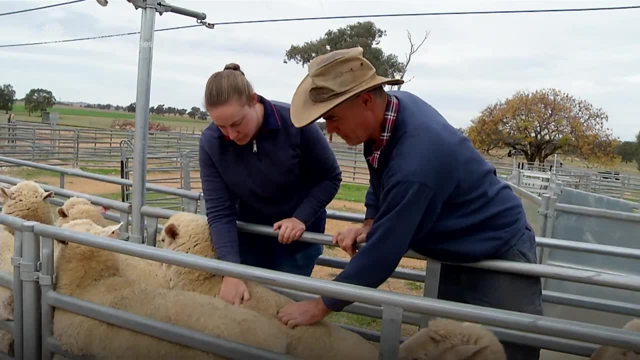 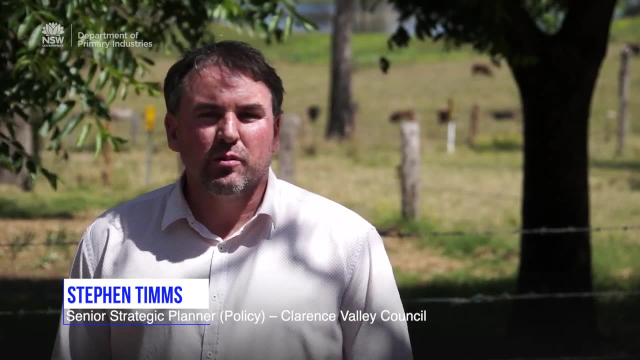 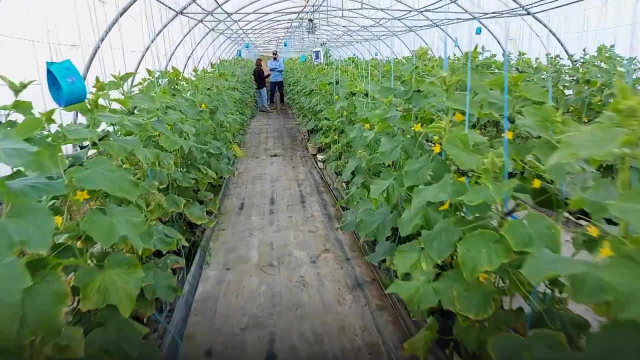 and guide agricultural land use planning policy in New South Wales. Clarence Valley has the largest agricultural sector on the New South Wales north coast, with one in four businesses identified as a primary producer. We recognise that a focus on continuing to support and nurture our agricultural industry. 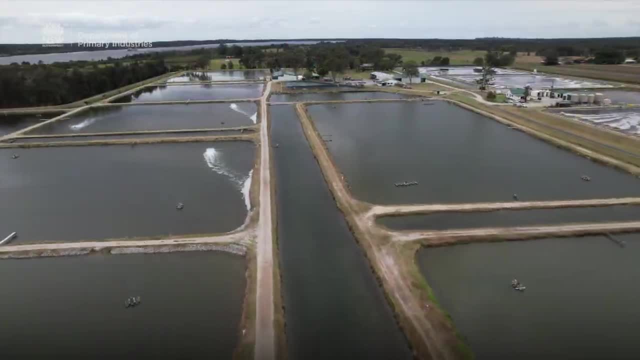 in all forms is critical to our prosperity. It is one of our key economic drivers. Part of our industry is the agricultural sector. It is one of our key economic drivers. Part of our industry is the agricultural sector. It is one of our key economic drivers. 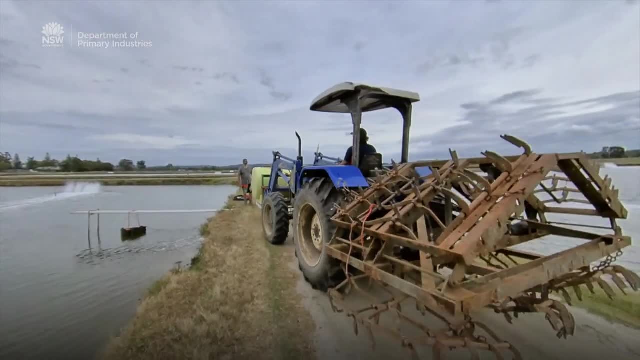 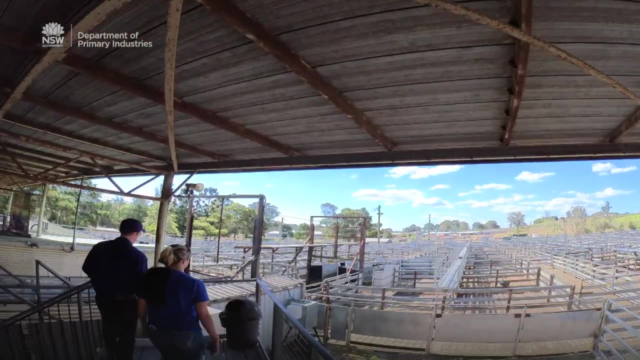 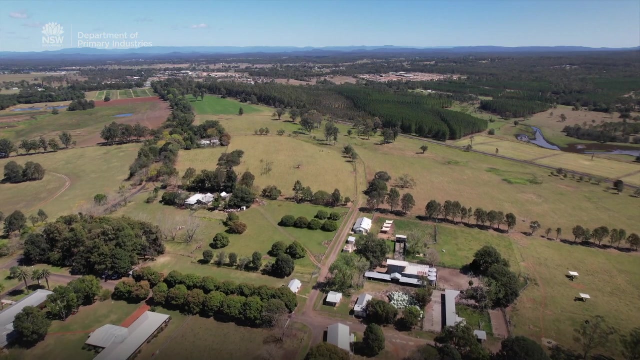 Our investment attraction is our capacity to support emerging and growth industries through protecting agricultural land from incompatible development and supporting infrastructure that supports our farmers- Things like the grafting cattle sale yards, fishermen's cooperatives and local markets. DPI's agricultural land use planning team have been really valuable in providing information. 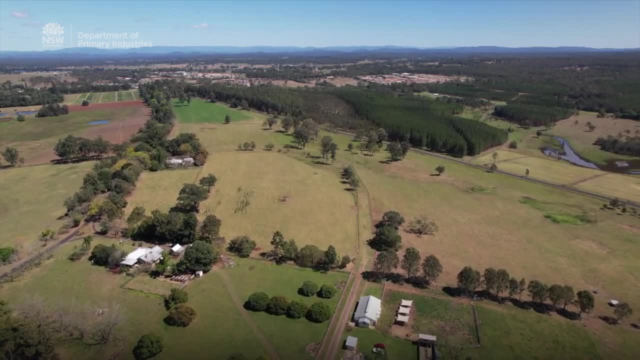 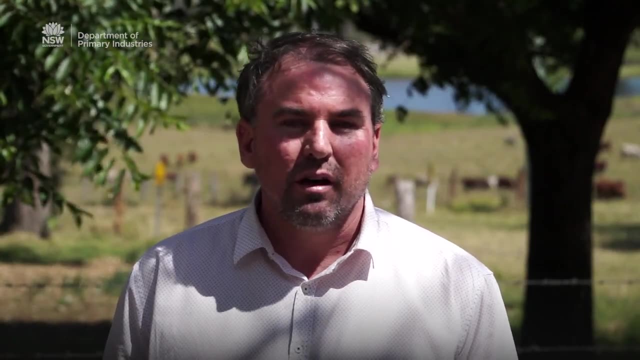 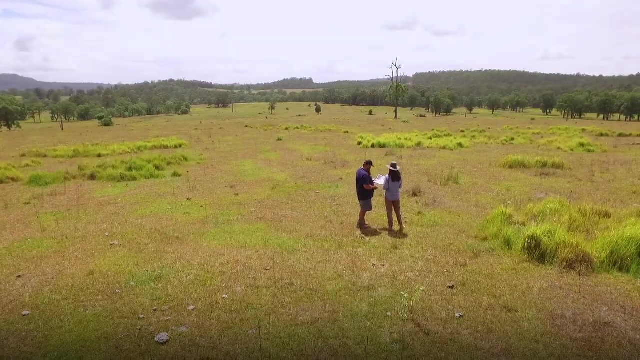 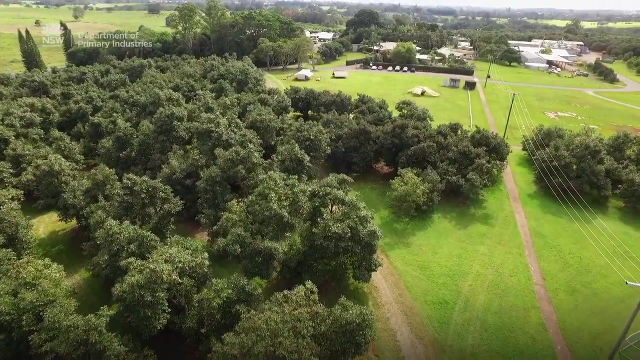 and support in the development of our local strategic planning statement and other strategic plans, and advice on planning controls and development. The agricultural land use planning team can provide advice for reducing land use conflict risk in rural and peri-urban areas. Land use conflict can arise between agricultural production systems or between agricultural 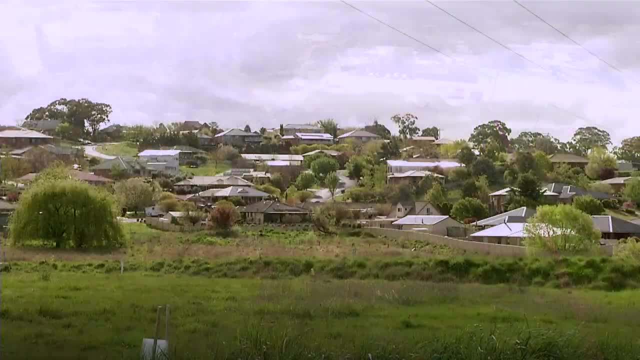 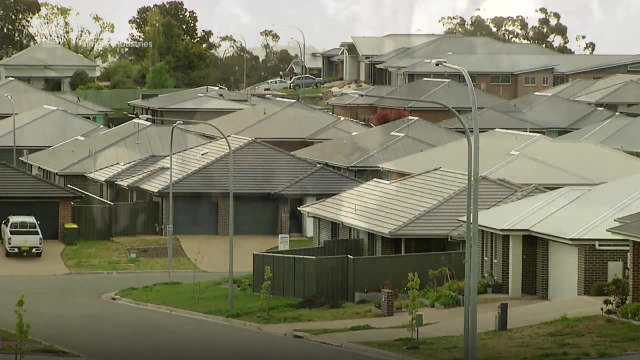 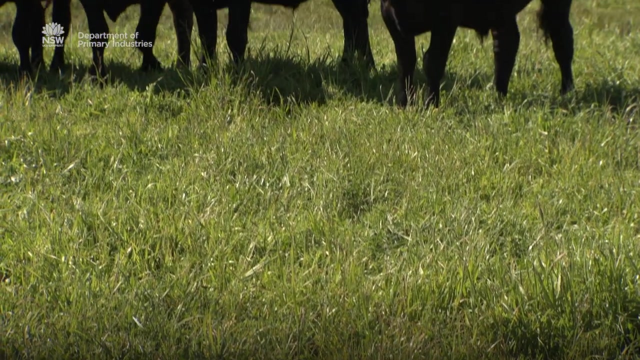 and non-agricultural land uses. Conflicts can have significant negative impacts on agricultural operations and the mental health of farmers or impacted residents. Land use conflict can be significant. It can be substantially minimised by good management of land uses, planning practices and expectations about farming activities. 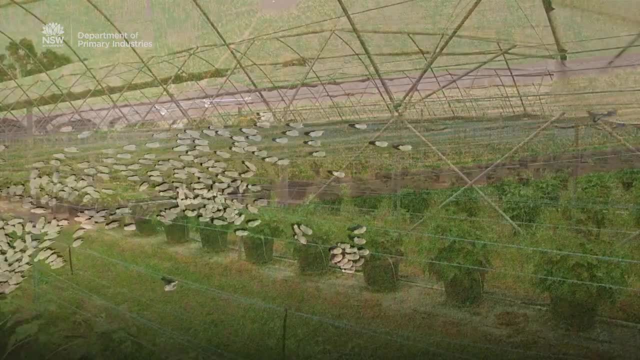 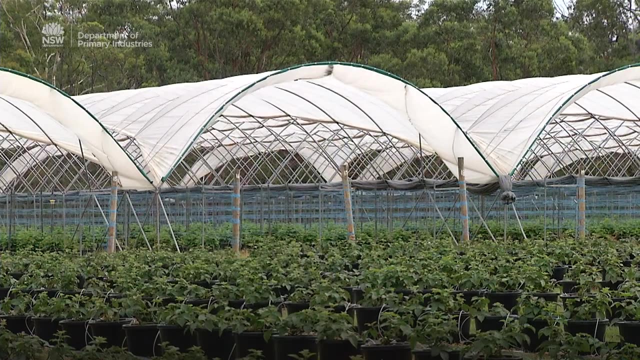 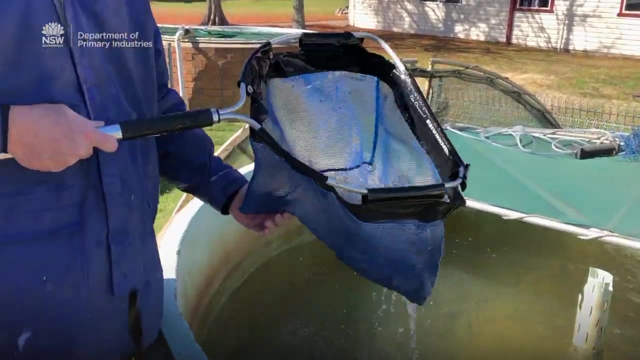 Agricultural practices are changing in response to a range of influences. Intensive agricultural practices are expanding across New South Wales and contributing to the growth in agricultural productivity. The agricultural land use planning team provide advice on intensive agricultural developments and can link councils and other authorities to industry resources and best practice management. 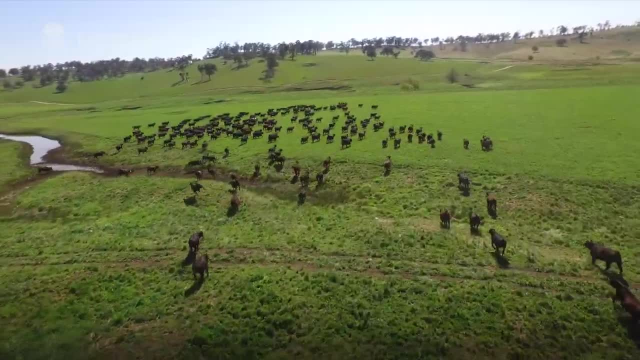 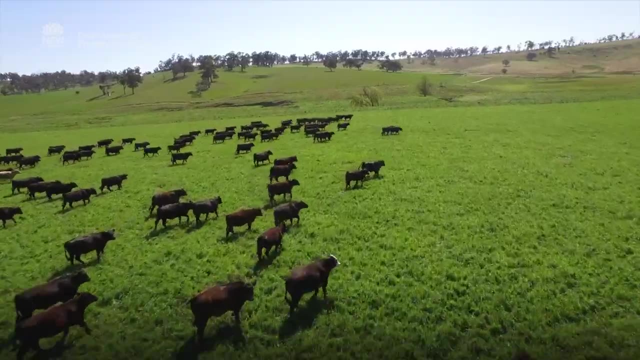 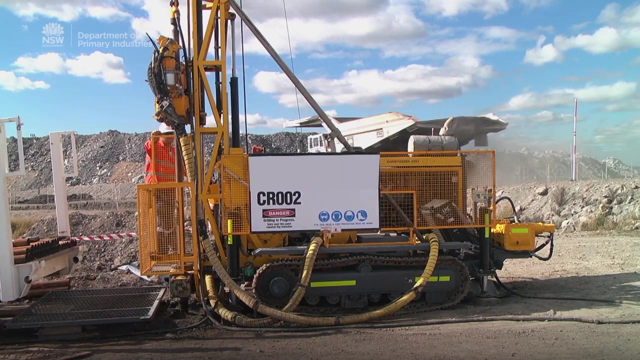 The team is working to deliver training and resources for local government and other planning professionals to support decisions on how intensive agriculture developments are integrated into the landscape and the community. The team also provides advice on major development projects that have the potential to impact on agricultural land resources or industries. 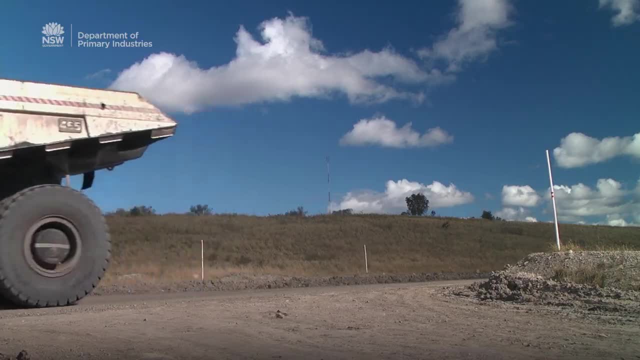 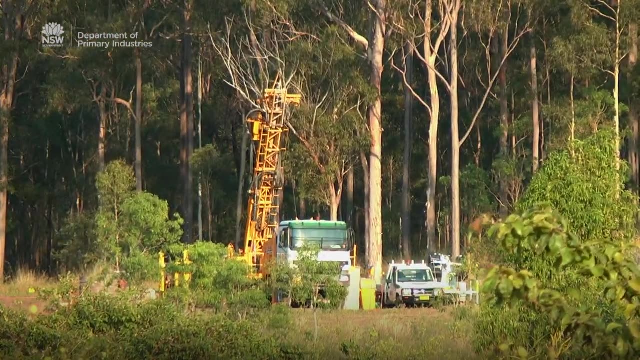 We seek input from technical specialists within DPI to consider the site suitability of the development and, where appropriate, identify measures that can be taken to improve the development of agricultural land. The team also provides advice on the potential risks to surrounding agriculture. The agricultural land use planning team can support local government in navigating diversification.